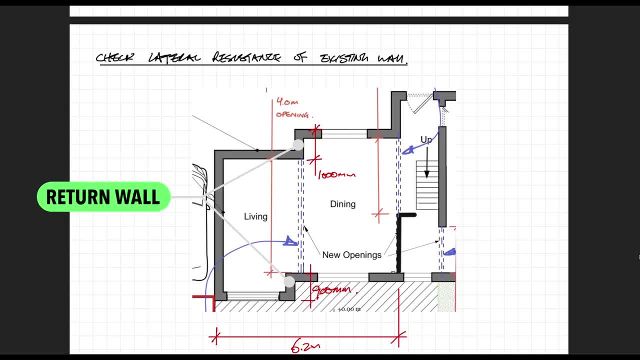 see there is a return or a kink in the external walls in both the north and the south elevation. what i'm going to be checking is to see if the return wall is strong enough to resist the lateral forces. if the return wall is strong enough, that means i won't need to check the external. 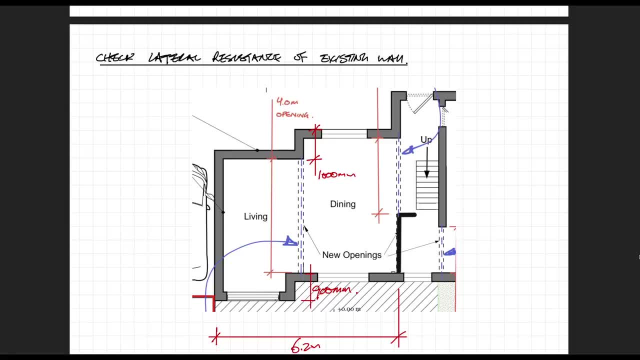 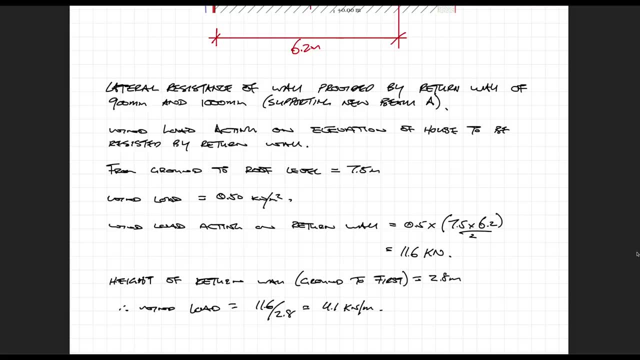 masonry panel as one really, really large panel. so what i'm going to do now is to calculate the force on this return wall. i'm choosing a wind load of 0.5 kilonewtons per meter square because the location of this house is within an area which is fairly sheltered, so the wind loads aren't going to. 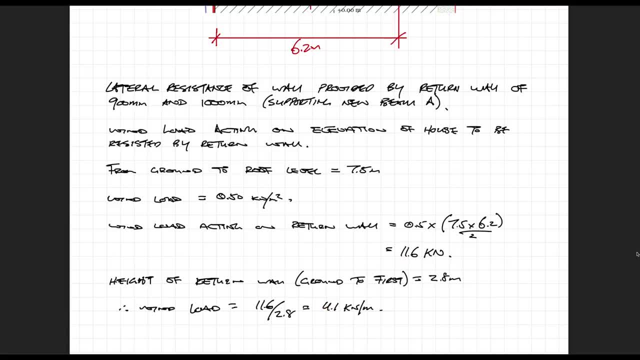 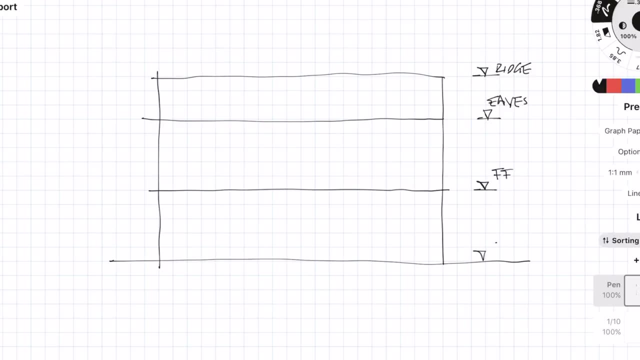 be that high, the wind load which you use will vary between locations, and if you're in a place which is very susceptible to high winds, such as an open area, or if it's an area on a hill, then the wind loads might be significantly higher, and this is something which you'll need to check separately. 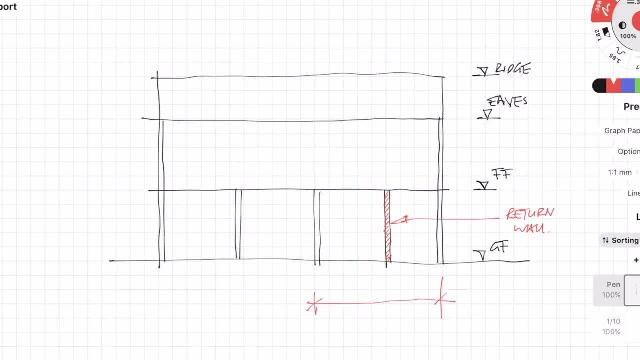 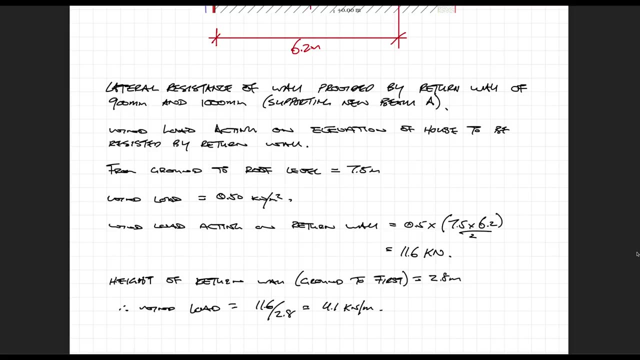 so all i'm doing is calculating the area or the tributary area of the elevation where the return wall is going to be resisting that force. once i've got the area, i can multiply by the wind load to get a force in kilonewtons, and then i can divide by the height of the wall and i end up with a. 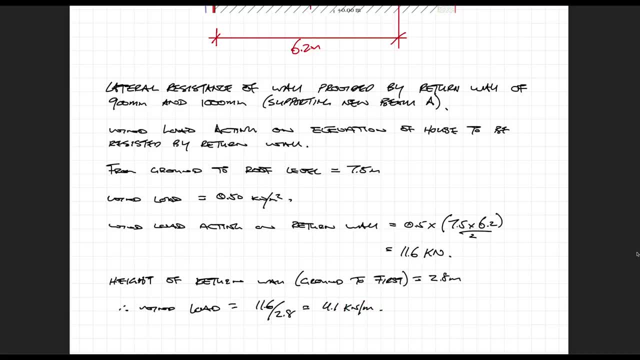 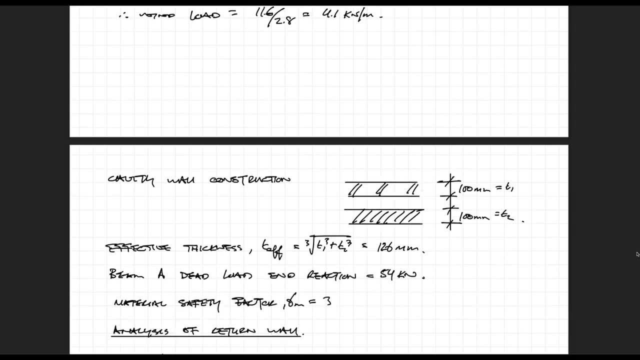 linear wind load of 4.1 kilonewtons per meter. the external wall is made up of a hundred mil block work, a cavity and a hundred milliliter of water, and a hundred milliliter of water and a hundred mil brickwork, because it's a cavity wall construction. that means our effective thickness. 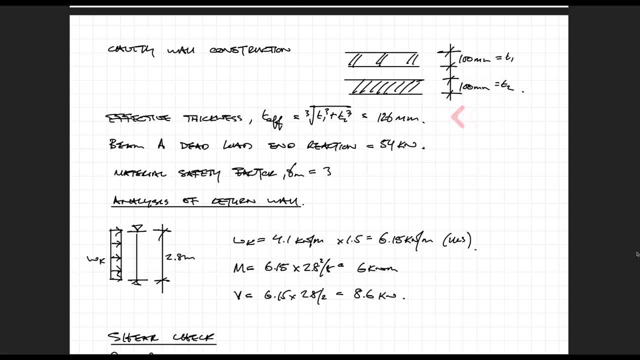 needs to be calculated, and that comes to 126 millimeters. i also mentioned earlier that this internal wall is supporting the floor and the wall above. from a previous calculation i would have worked out the beam's end reactions and i would have had a dead and alive load. 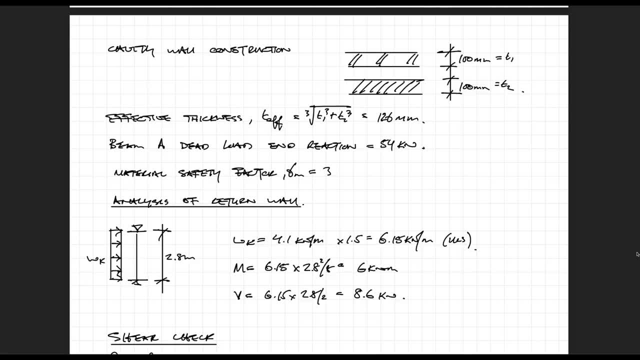 because the gravity load actually benefits or enhances the resistance of the wall. i'm only going to consider the dead load and ignore the live load completely, and i'm going to be using a material safety factor of three. we can do a quick 2d analysis and work out the bending. 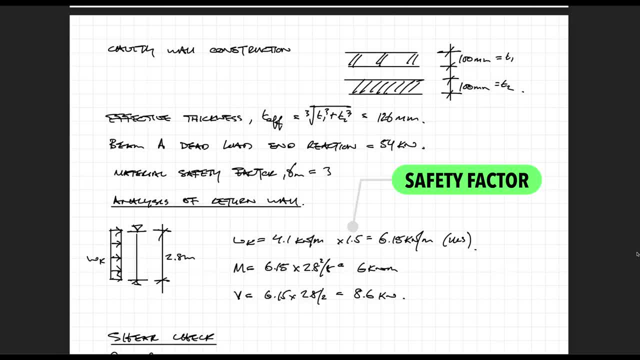 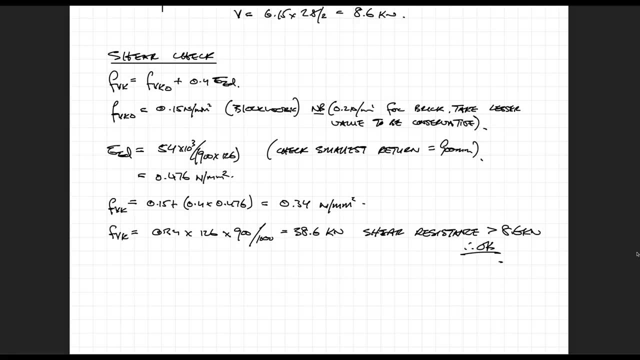 moments and the shear force. so i'm going to do the shear check first. the shear resistance is defined as fvk and that's equal to fvko plus 0.4 for design stress. fvko is the characteristic initial shear strength of the masonry. typically for block work it's 0.15 and brickwork is 0.2 to. 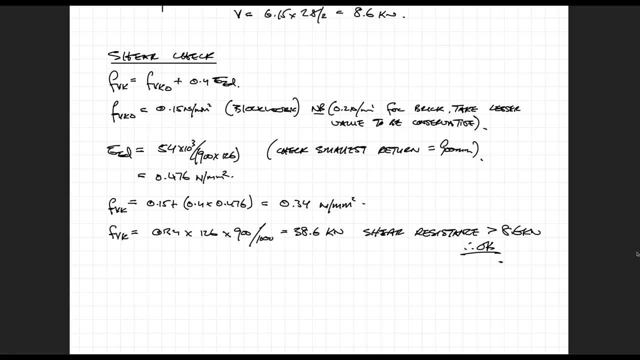 be conservative, i chose 0.15. i'm going to be checking the smallest return and that return length was 900 millimeters. so to work out the design stress, i'm going to take the beam end reaction, which was 54 kilonewtons, and divide by the area of the masonry pair, and that gives me a. 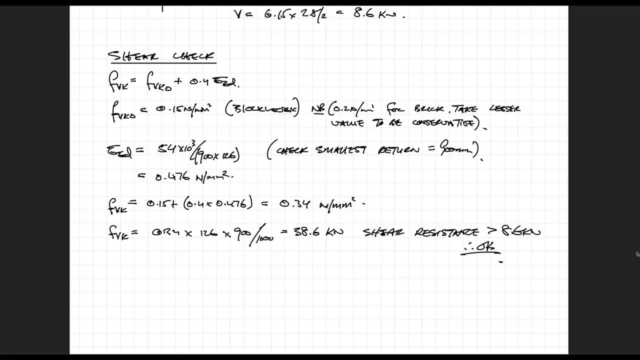 stress of point four, seven, six newtons per millimeter squared. so now i can add this value to Spanish, to 0.15, and get a design shear stress of 0.34 newtons per millimeter squared, which equates to a shear resistance force of 38.6 kilonewtons. This shear resistance is greater than the. 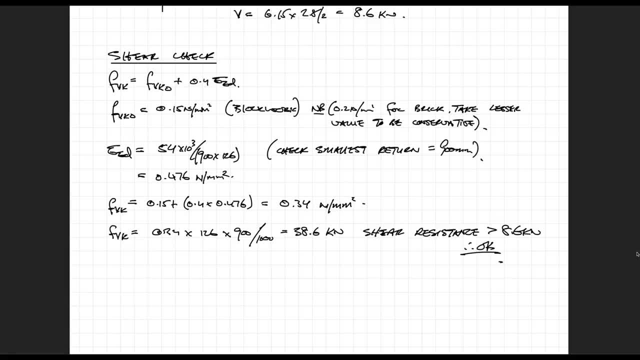 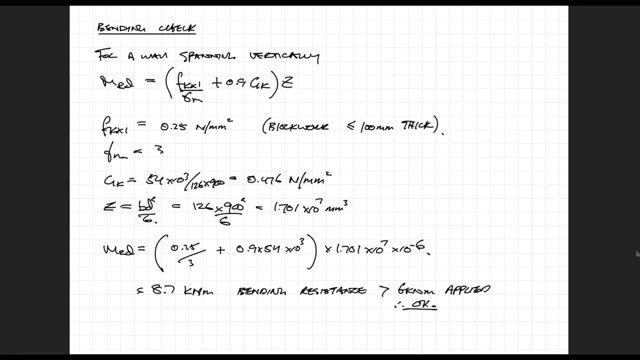 shear force applied. therefore, the design check has passed. Okay, so now moving on to the bending check. now, for this example, the wall is going to be spanning vertically, and when a wall is spanning vertically, to check the bending moment resistance, we need to use this equation: Fkx1 is simply the 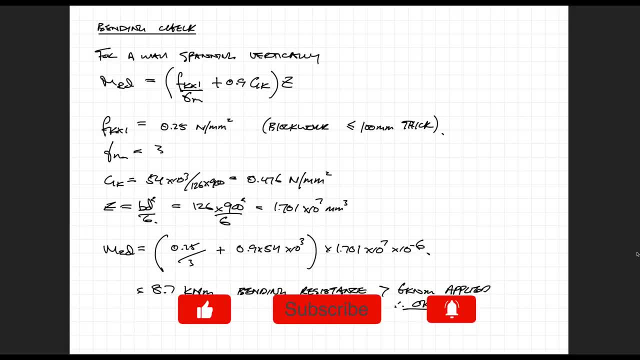 characteristic flexural strength of the masonry, and this varies depending on what type of masonry you're using. In this case, we're using a value of 0.25 newtons per meter squared, because our block work is equal to 100 millimeters thick. Gk is still the actual stress due to dead load and z. 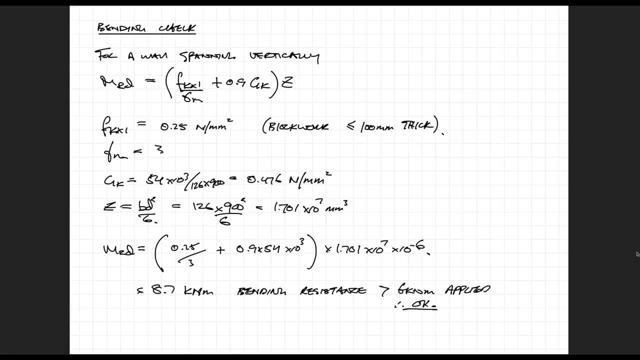 is the section modulus. The stress is calculated in the same way as we did in this shear check and the section modulus is calculated using bd squared over 6, where b is 126 and d is 900 millimeters. Plug all these numbers into the bending moment resistance. 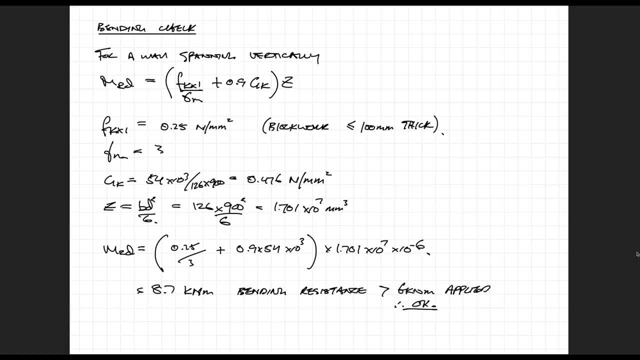 equation above and we get a resistance of 8.7, which is greater than the applied, which was 6 kilonewton meters. Therefore our check passes and therefore we don't have to do a separate check on the entire masonry panel, therefore saving us a lot of time.